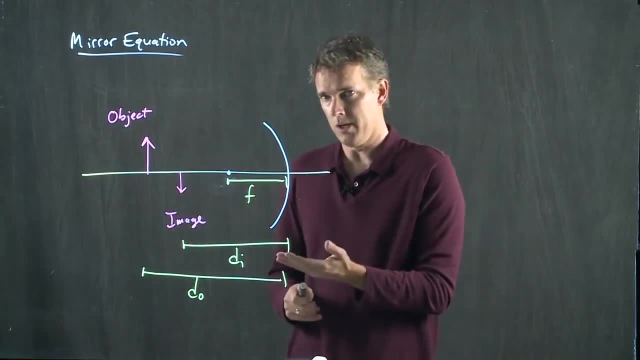 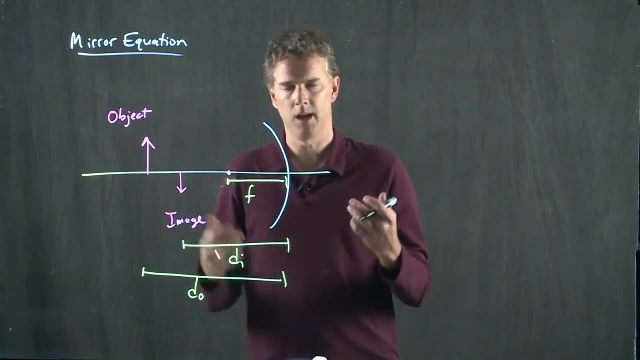 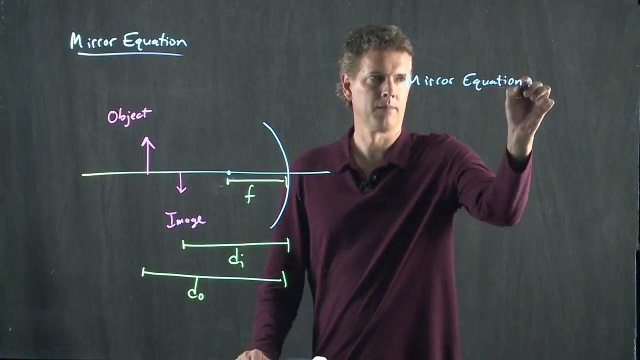 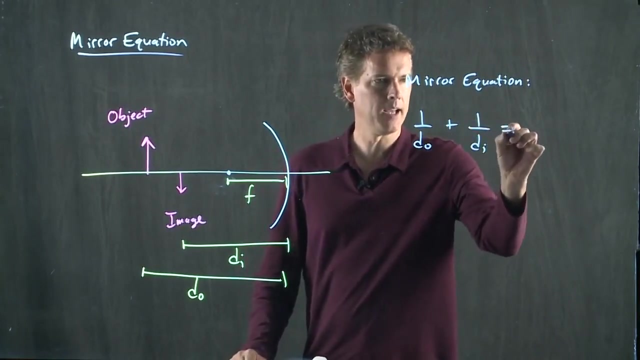 All right. So the mirror equation allows us to determine where that image is going to be located, And the mirror equation is the following: One over d O plus one over d i equals 1 over F. First fraction, Second fraction, Third fraction. 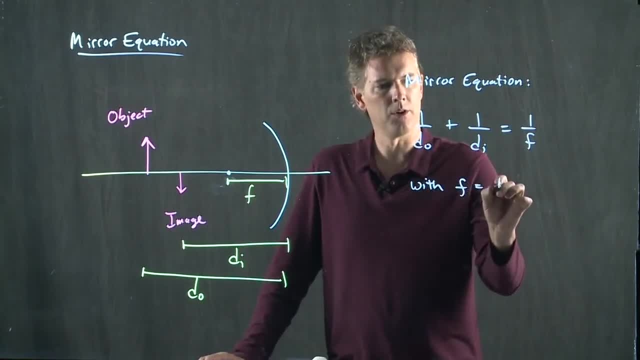 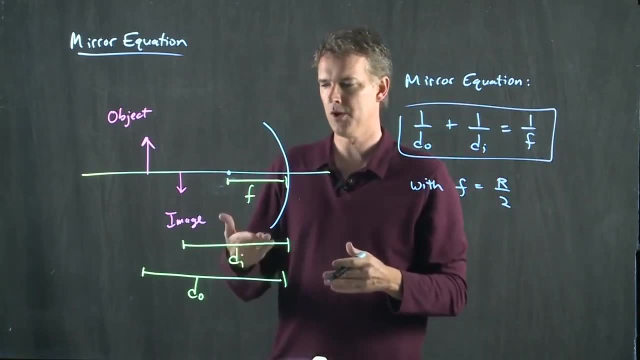 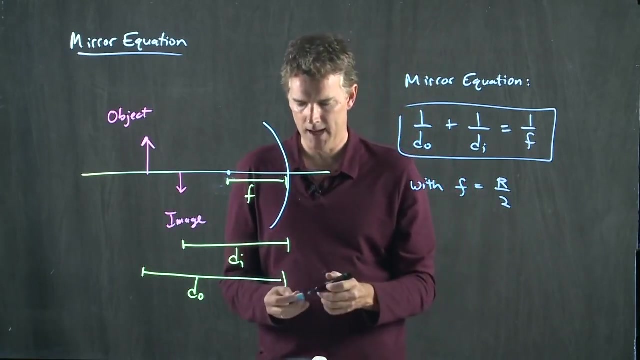 Fourth fraction. Fourth fraction. Fourth fraction. Fifth fraction. Fifth fraction: that f was equal to r over 2.. This thing is going to help you determine where di is. So let's take a look at the last clicker question that we just looked at and verify that this equation is. 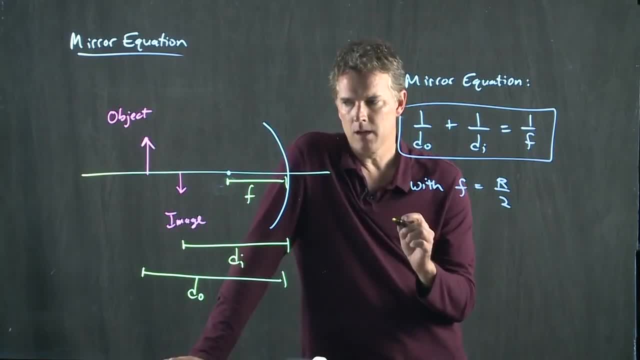 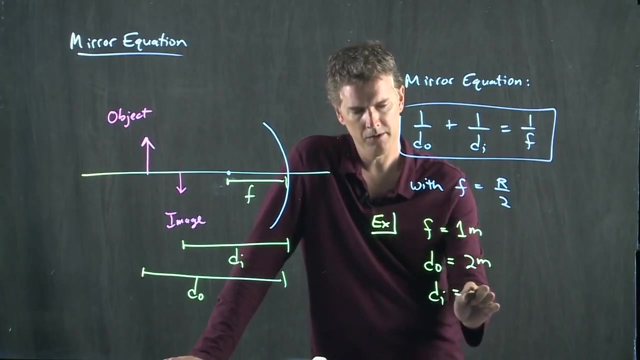 in agreement with that. In that equation we had the following: We had that the focal length was 1 meter, But we also had that do was 2 meters. Can we solve this now for di? Well, yeah, that doesn't look too bad right. 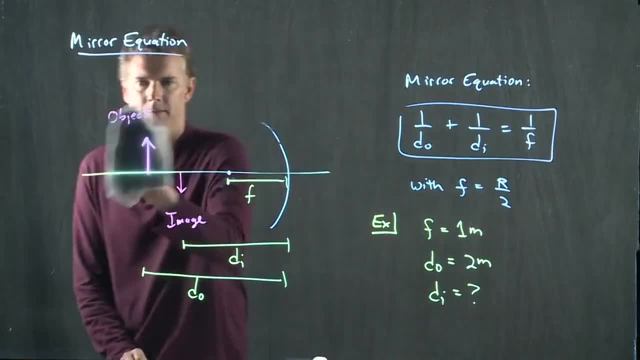 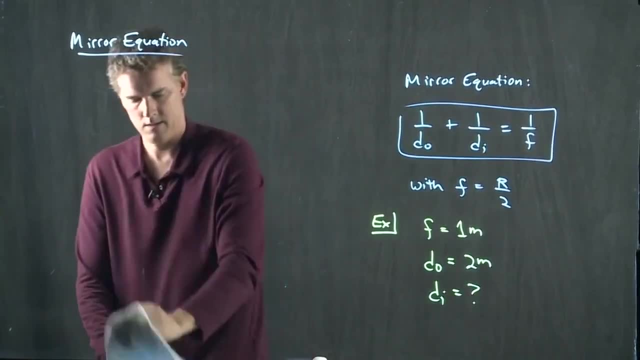 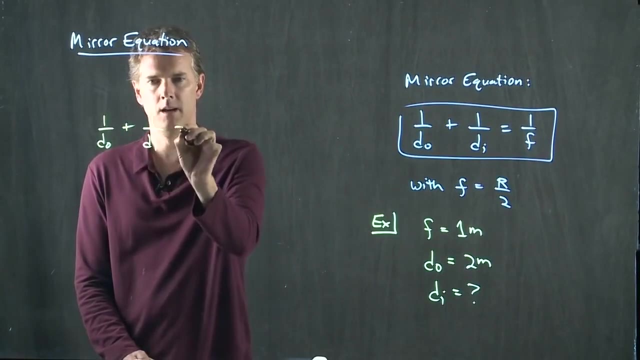 Let's take this equation and let's solve it for di. So we're going to take this equation and let's solve it for di. So we're going to take this equation and let's solve it for di. All right, so we've got 1 over do plus 1 over di equals 1 over f. 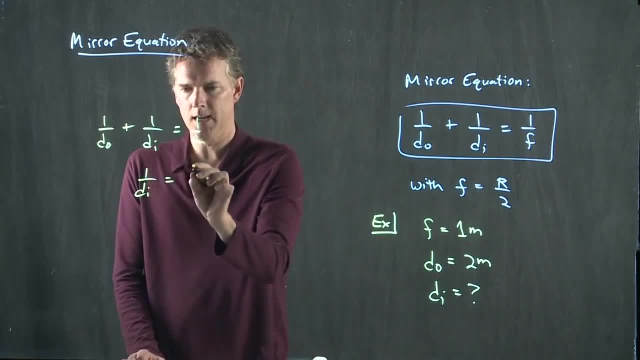 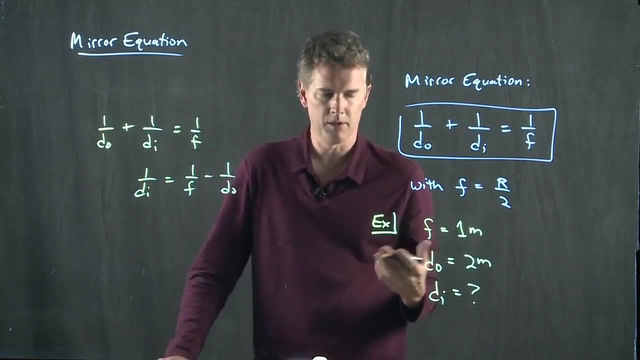 So let's move the do to the other side. I got 1 over di equals 1 over f, minus 1 over do, And now I know all those numbers so we can just plug them in: 1 over di equals 1 over f. 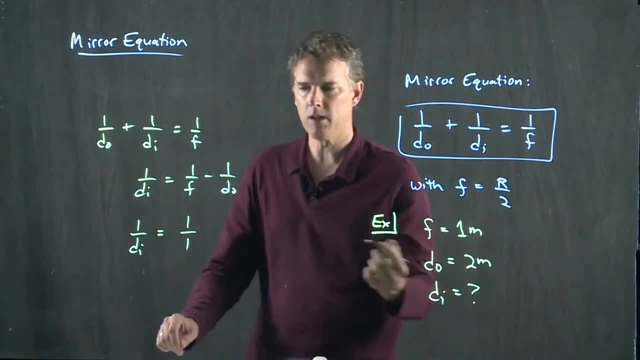 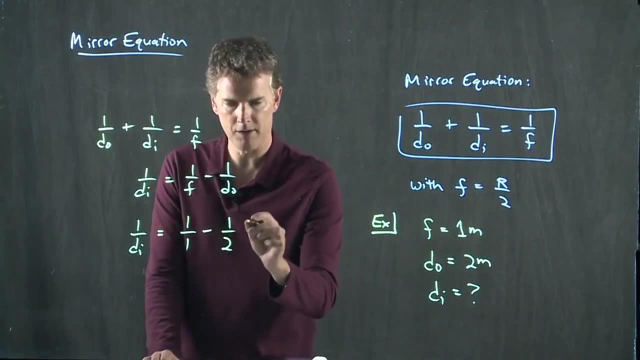 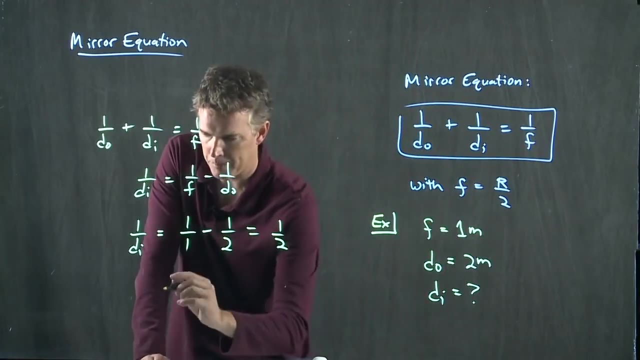 Which is 1 over 1 minus 1 over do, which is 1 over 2.. All right, 1 minus 1 half is 1 half, So 1 over di is equal to 1 half, And if I flip it back over I get di is equal to 2.. 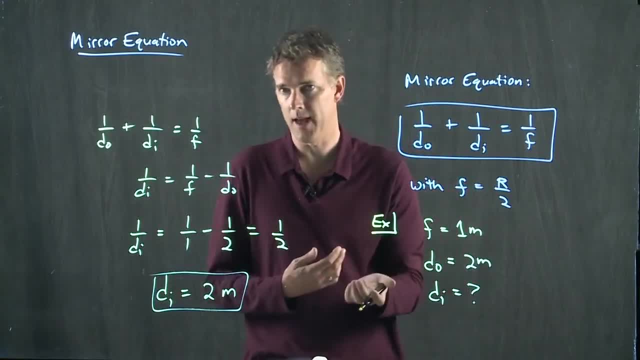 And that's exactly what we found on that picture a second ago. If the object was 2 meters from the top, then it would be 1 over 2.. If the object was 2 meters from the top, then it would be 1 over 2..